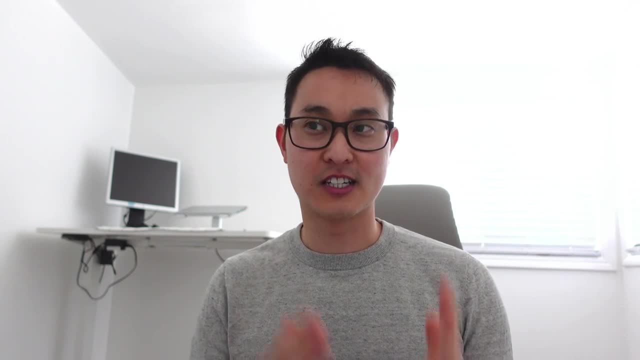 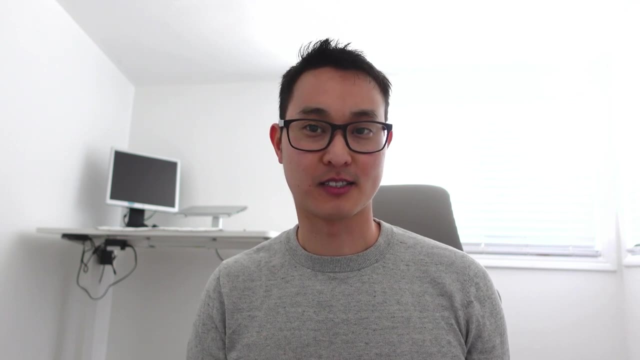 field. in order to be successful, You just need to be good enough to pass those classes at your university. So, for example, I don't use calculus or advanced math on a daily basis at my job. Honestly, I haven't even touched calculus since college. So if you're worried about being bad at math or it being the 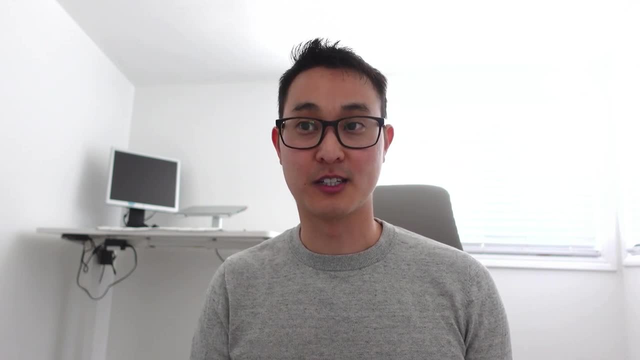 stupidest one at the university. No, Always get research done. Use them at the highest Fujifilm level. I just want to include a fewоки, but then stop by the lab in conditions where it's really interesting, being the reason why you don't go into this field. just don't worry about it. math is not your main. 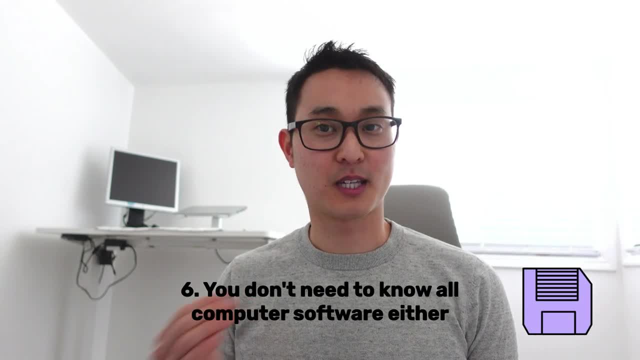 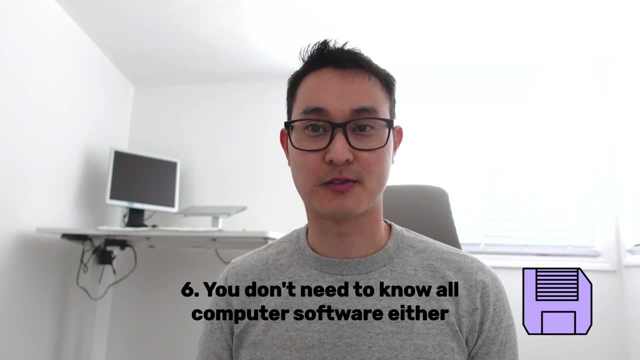 priority as an environmental engineer. six, piggybacking off of the previous point, you don't need to be an expert in gis, autocad or any other computer software either. some of these computer programs may not even be applicable to your day-to-day job. it all depends on your responsibilities. 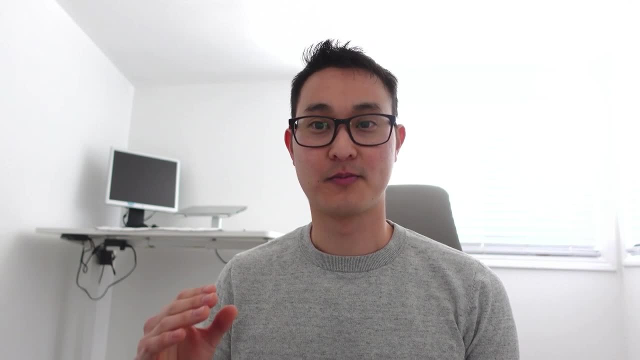 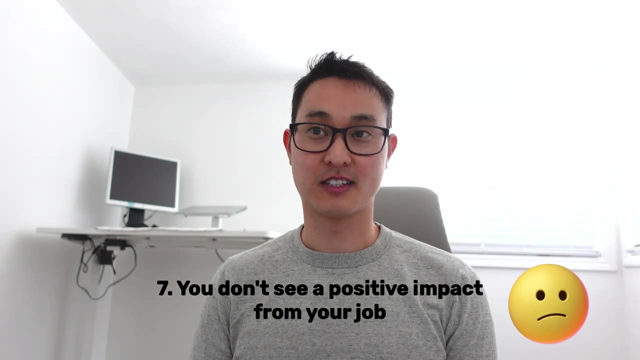 and job description, but it will tell you when you apply for a job what you need to know to be good at all is to say, not everything you learn at school will be used at your job. seven: this is going to be a tough pill to swallow, but you don't see the impact of your job. yeah, i know many of you. 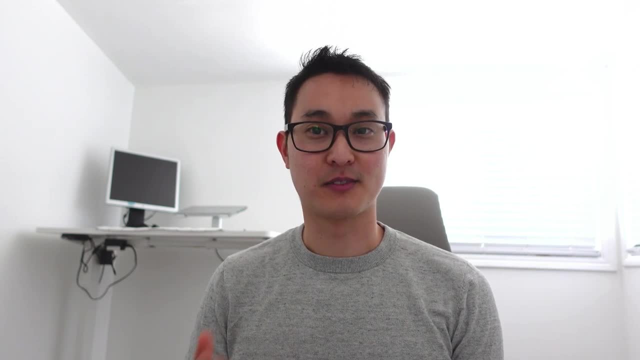 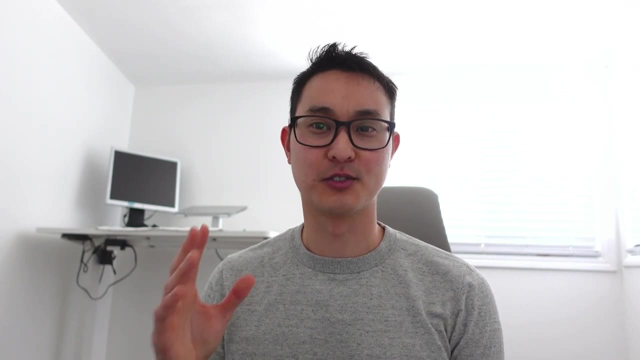 watching were like me during my student years. we wanted to make a difference in the world, so that's why we decided to pursue environmental engineering in the first place. however, it's not as visually impactful as you'd think. you don't see the drastic change in the amount of pollution around the world. 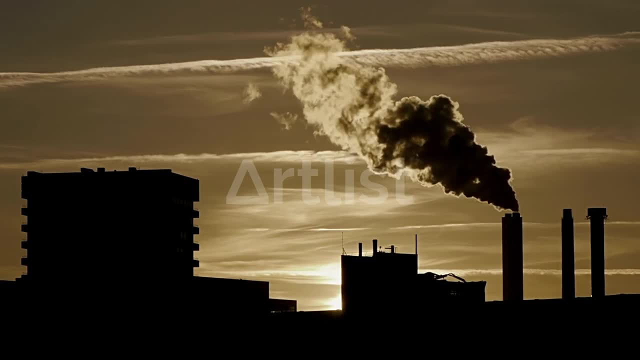 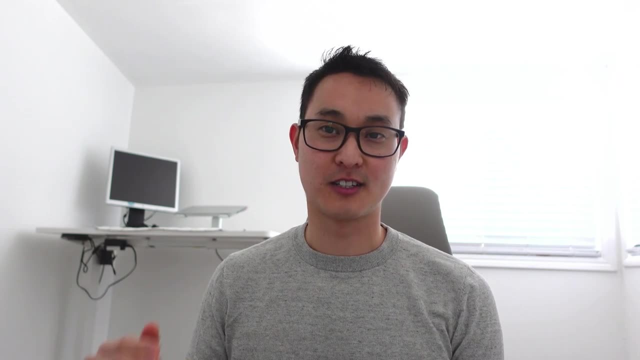 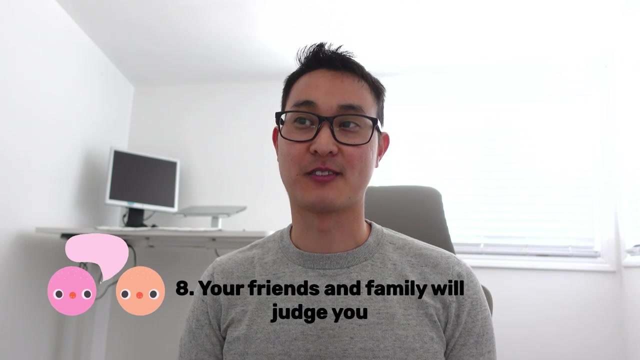 or you see your research being implemented or adopted and accepted quickly, globally, by all industrial facilities or politicians. it's sad to say, but change is slow, if it's even accepted in the first place. number eight: your friends and family are going to judge you based on the fact that you're pursuing this field. so if you're asian, like me, your family 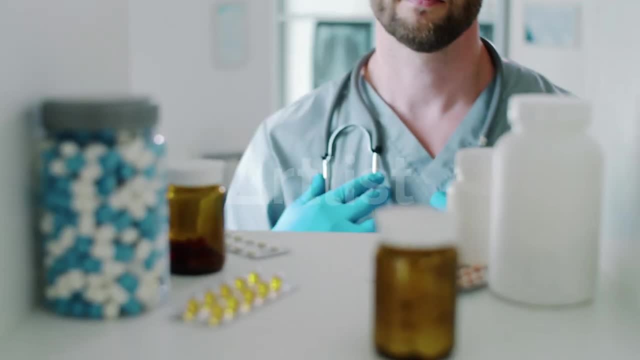 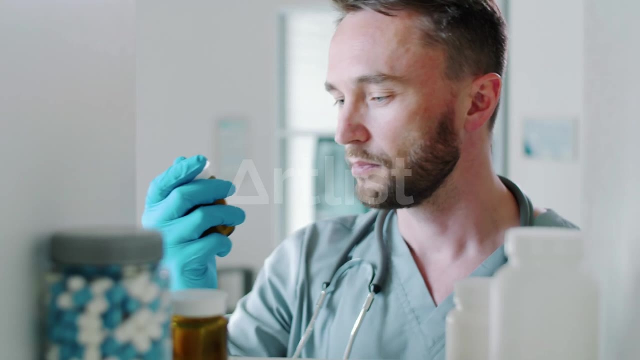 probably doesn't agree with your decision. they wanted you to go towards, like the medical route, right, but i mean that's easier said than done. deep down you know you wouldn't enjoy listening to them or going down the medical field anyway, so don't let them force their 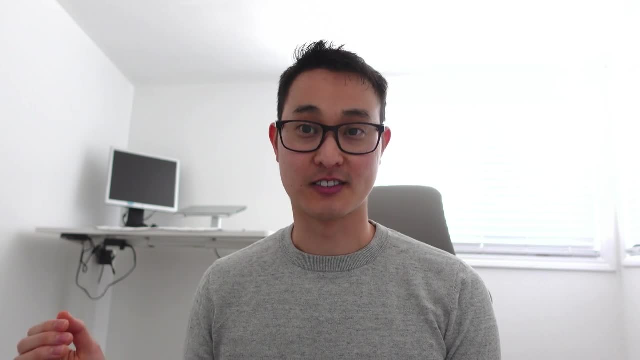 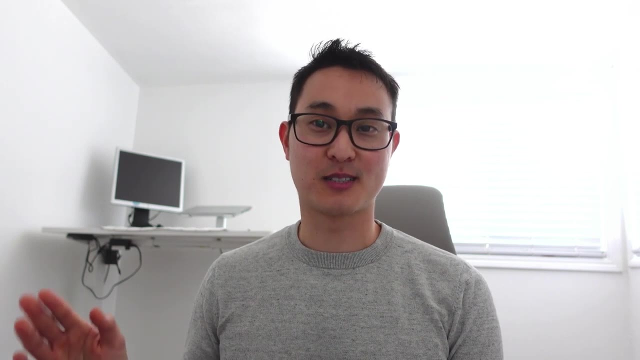 expectations on you. it's your life, not theirs. nine: you're probably going to be working at a desk in an office like 80 of the time, so if you're expecting to be exploring, like the amazon jungles, or seeing lots of greenery, you're probably thinking of a different job, although environmental.